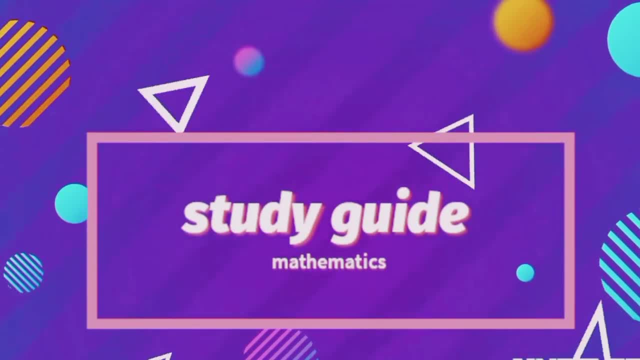 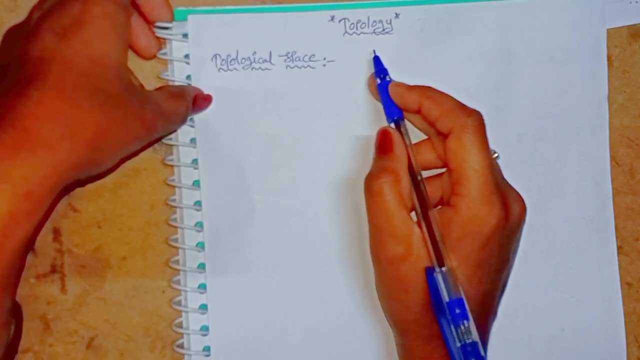 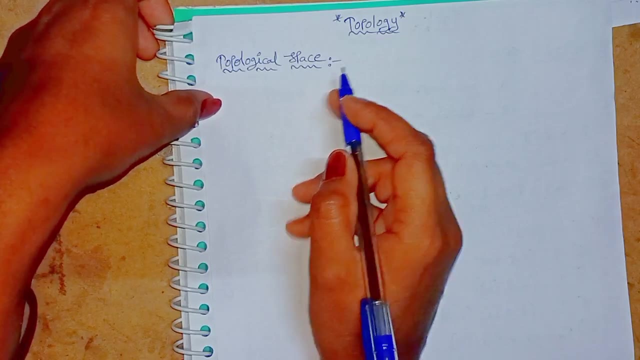 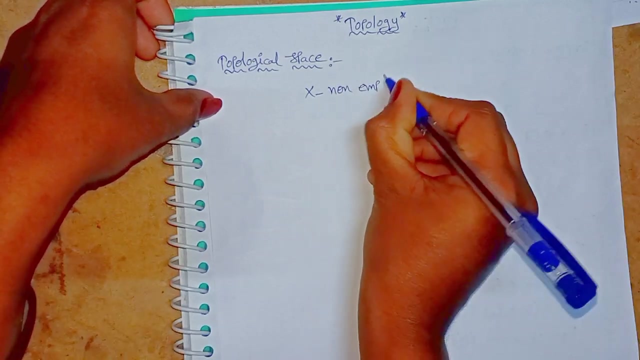 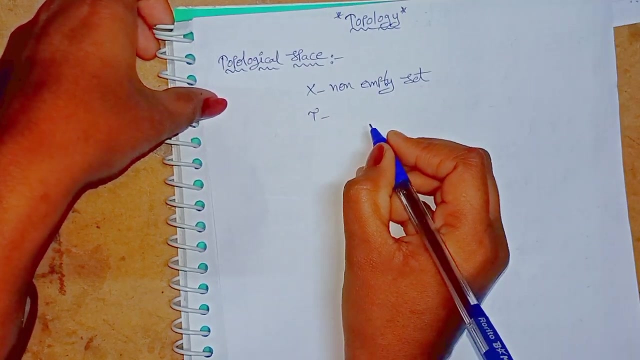 Hi students, I am Swati, So here. topic: topology, which is the most important MS standard here: theorems, definitions, example, Okay, topological space. What is the meaning of topological space? Let us consider: x is any non-empty set, x is any non-empty set and tau, Tau be a collection of. 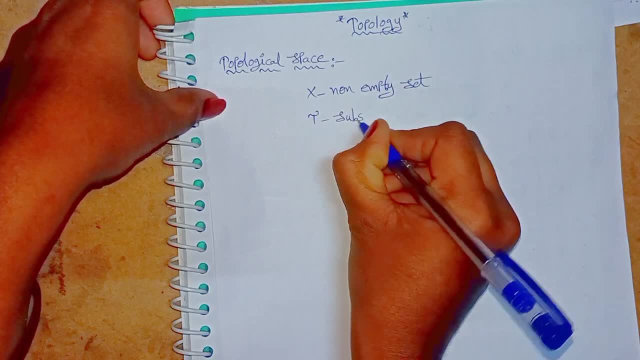 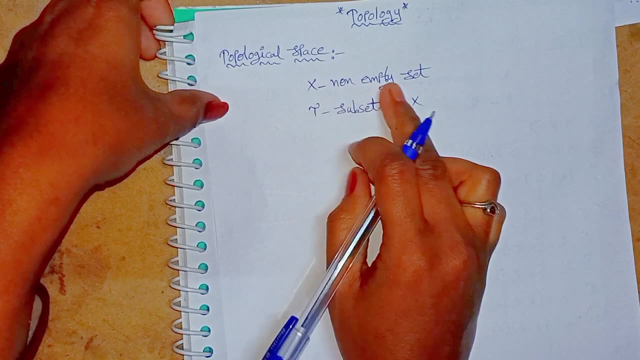 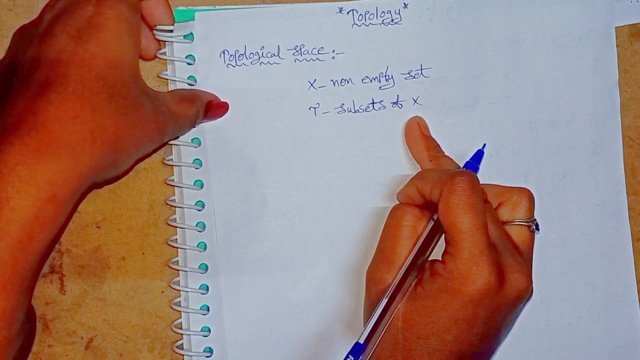 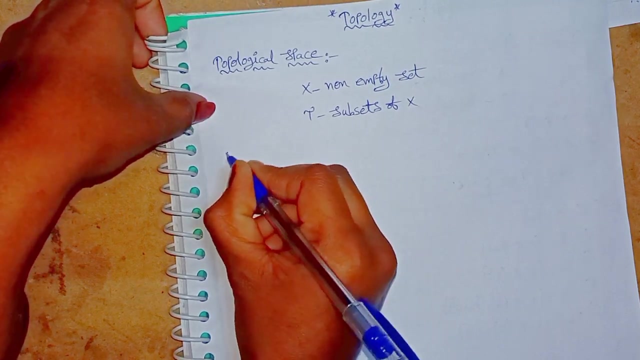 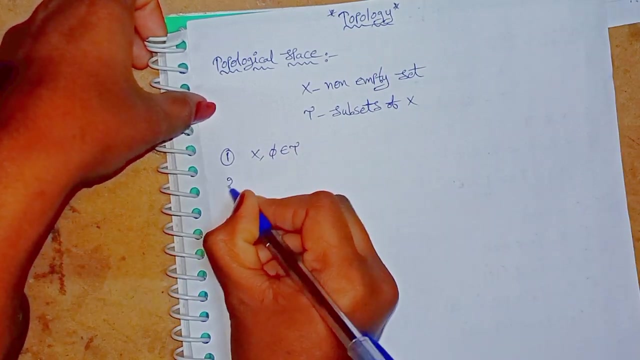 subsets of x and tau be a collection of subsets of x. x is a any non-empty set and tau be a collection of subset of x. x is set to be topological on x If it is satisfies the following three conditions. First condition: x comma pi belongs to tau. Second condition: we have to consider two sets. 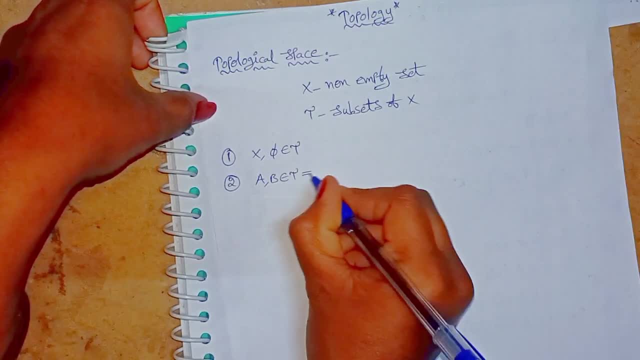 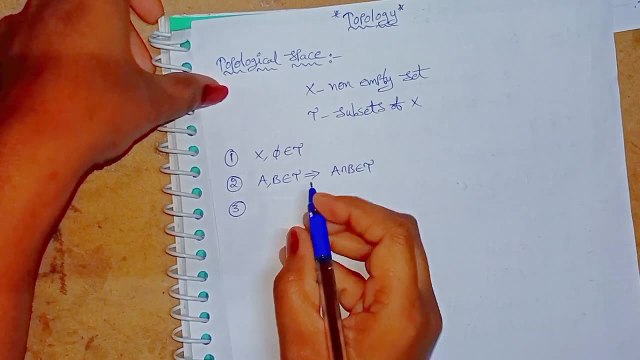 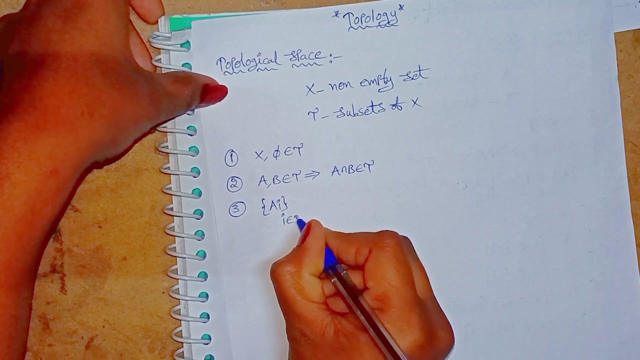 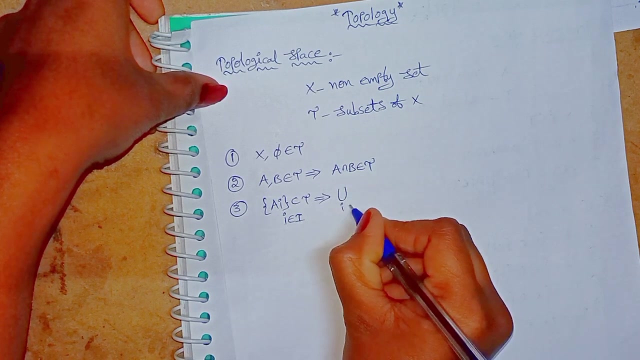 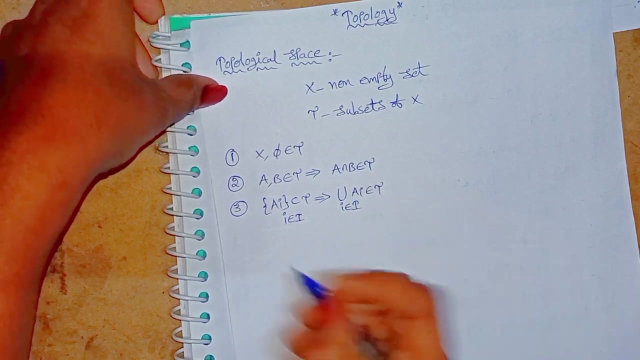 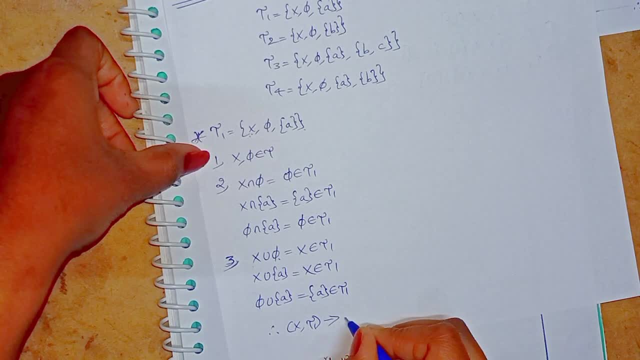 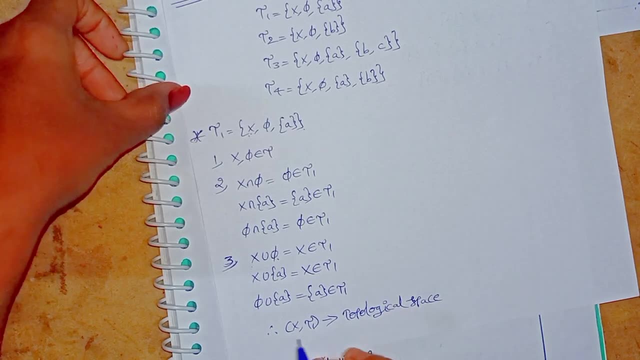 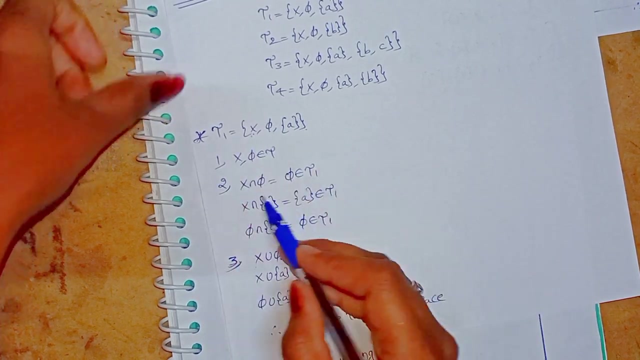 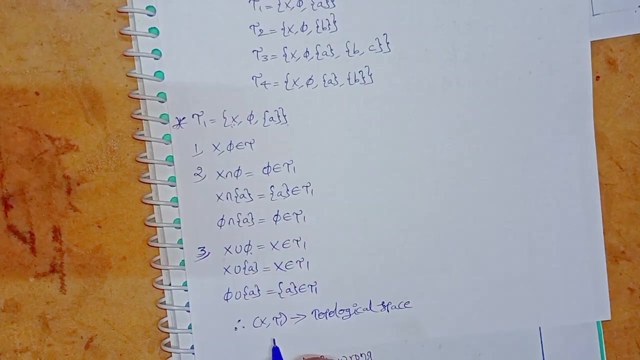 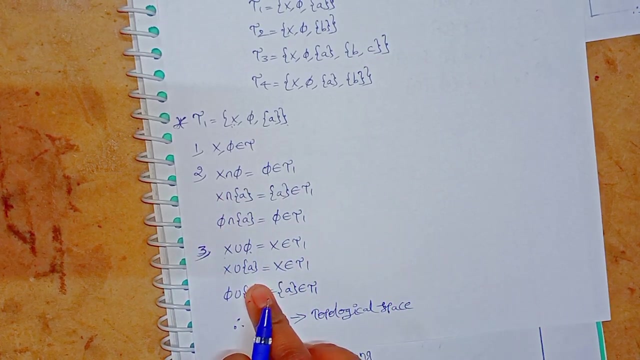 tau 1 is a topological arm space. x comma. tau 1 is a topological space. x intersection, pi, x intersection. pi is also in tau 1. x union is also in tau 1. x comma. tau 1 is a topological space. here we considered intersection, here we considered union, here we satisfied three. 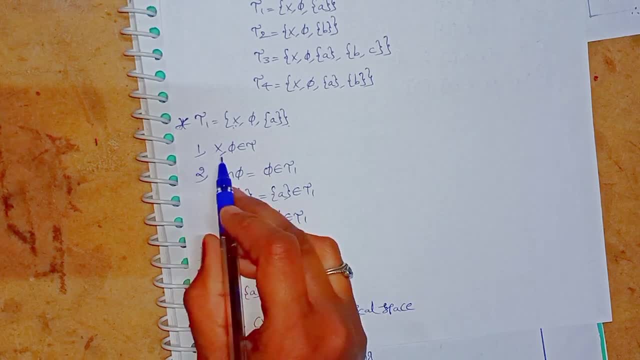 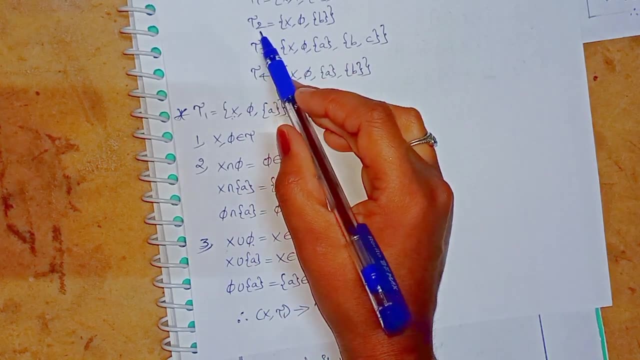 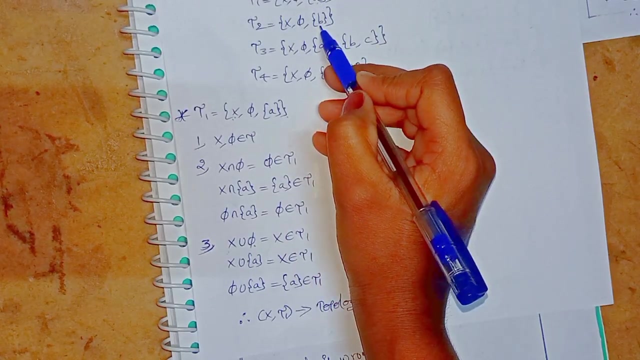 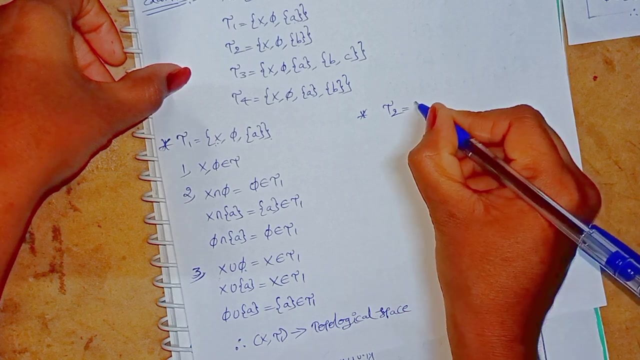 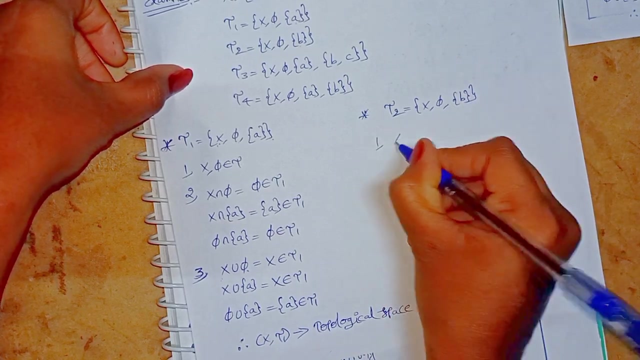 conditions. first condition: algebra structure: x comma, tau 1 is a topological space, as the second one, tau 2, pi comma single term b. here single term a, single term b: same tau 2 equals to x comma, pi comma single term b. first condition: x comma pi belongs to tau 2, clear. 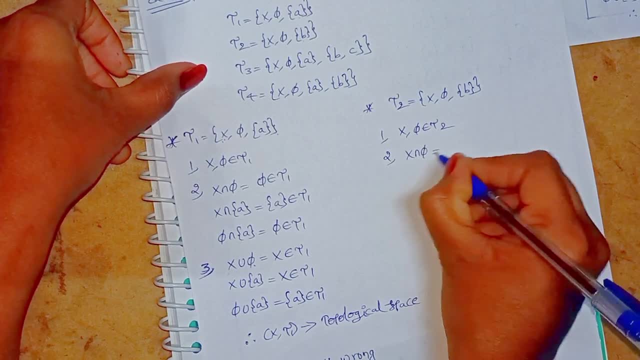 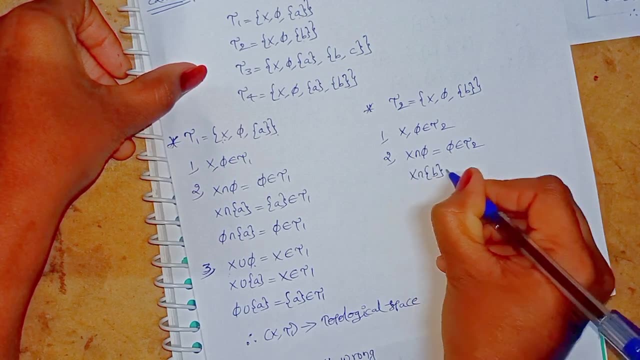 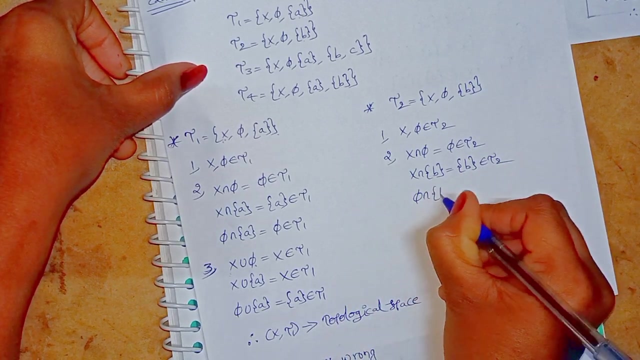 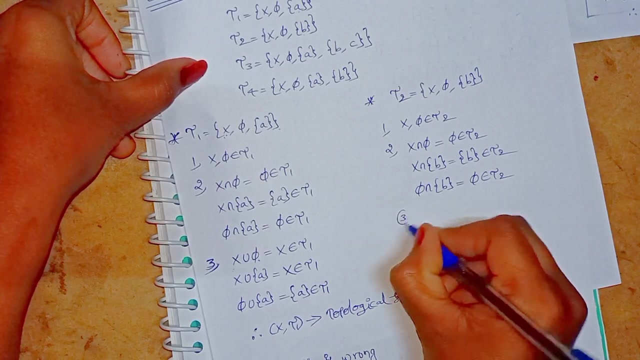 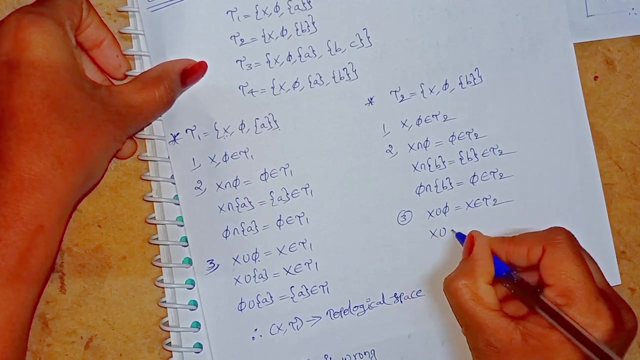 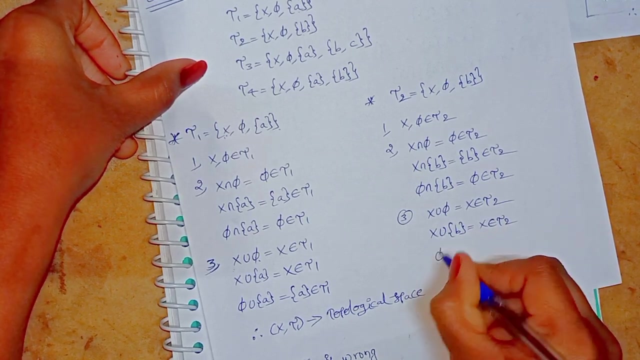 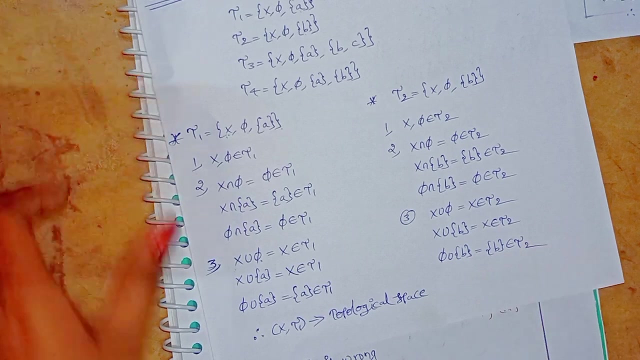 x intersection pi. pi belongs to tau 2. x. intersection: single term b. single term b belongs to tau 2. pi intersection: single term b equals to pi belongs to tau 2. third condition: x union, pi equals to x belongs to tau 2. x. union b: single term b equals to x belongs to tau 2. pi union: single term b equals to single term belongs to tau 2. 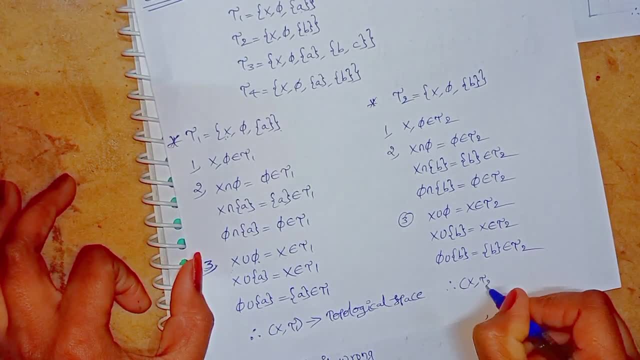 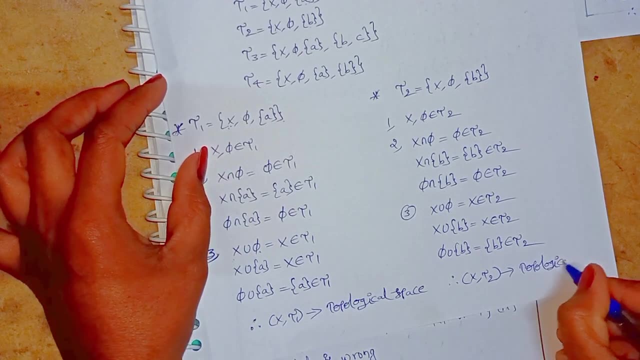 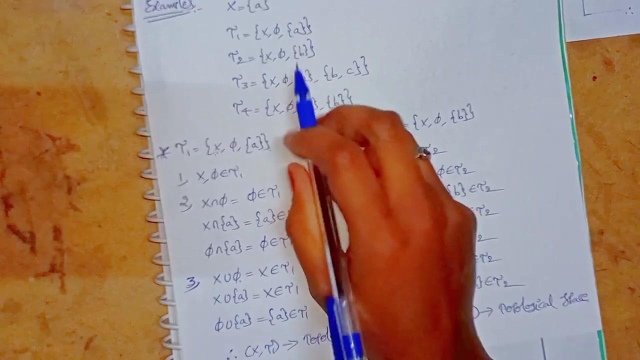 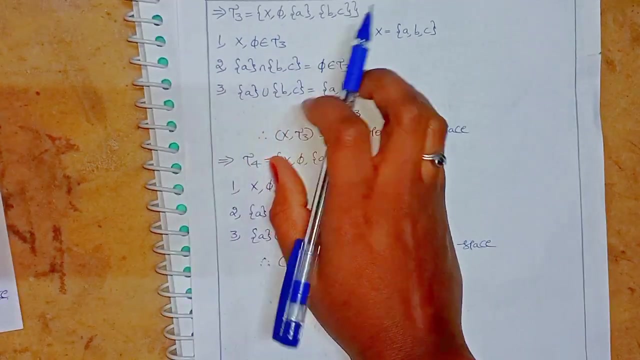 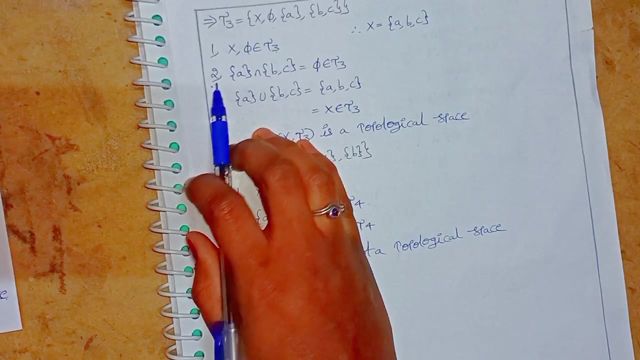 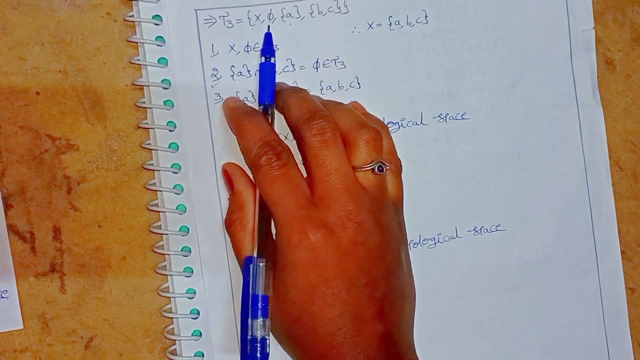 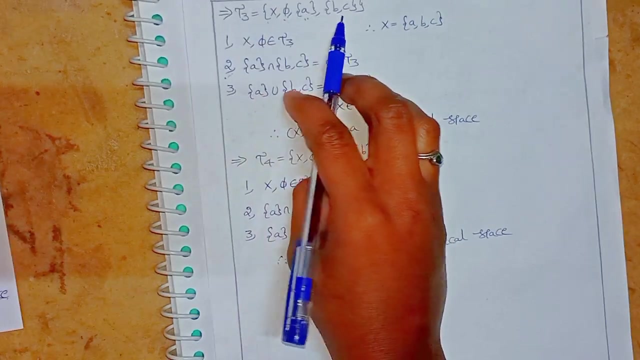 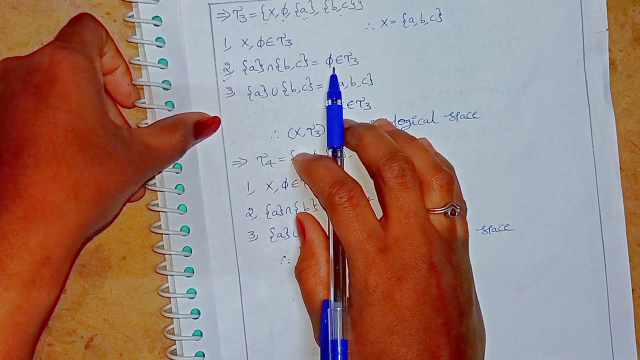 the algebra structure: x comma, tau 2 is a topological space. is a topological space. okay. third one: tau 3 equals to x comma pi. single term a, b, comma c. first condition: x comma pi belongs to tau 3. second condition: x intersection, pi equals to pi. x intersection single term equals to single term a, pi intersection: single term a is equal to pi. next single term: intersection b, comma c. single term: intersection b, comma c equals to pi. comma pi belongs to tau 3. 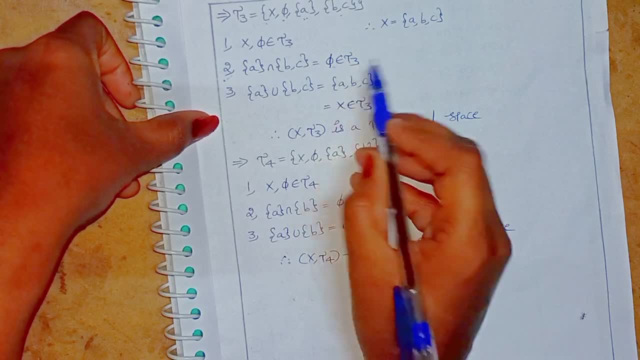 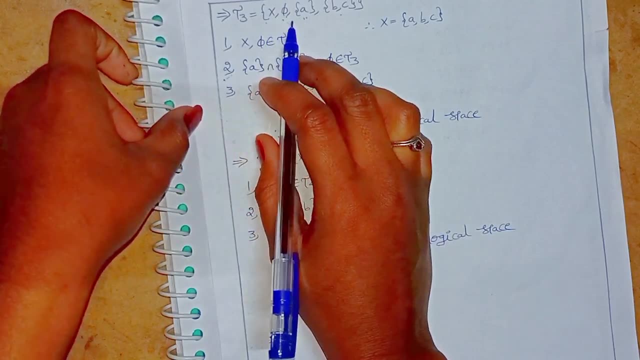 third condition: x intersection pi equals to pi. x intersection single term: b equals to tau 3, pi belongs to tau 3. next condition: 然後akiец condition. that's how we find 0.99 girl: x union pi equals to x. next function: x union pi equals to x. 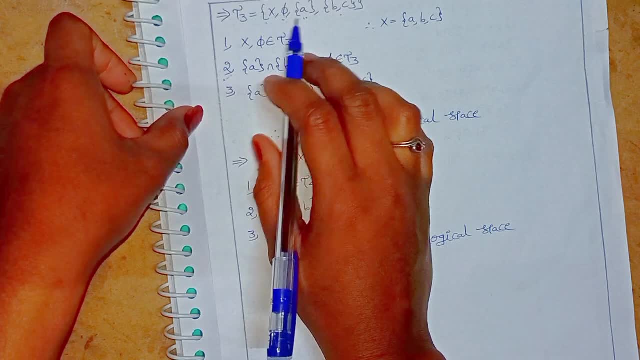 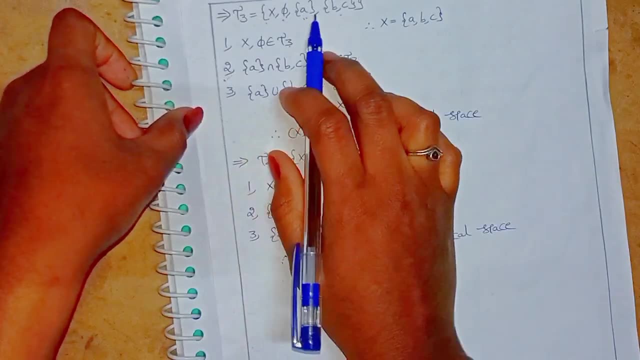 eme x union, single term equals to x. that's how we find 0.99 girl. x union pi equals to x belongs to tau 3 premiersung unihi as loss union. as loss arribe, as loss bouger. Split our a using 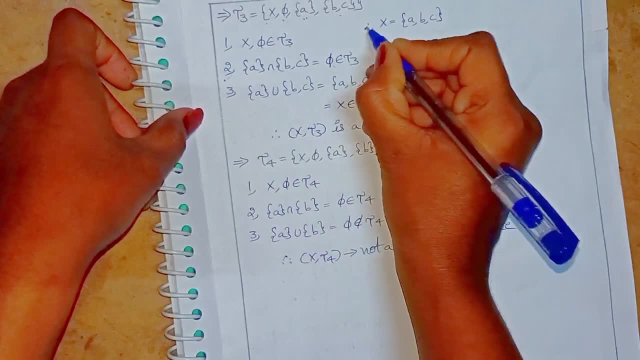 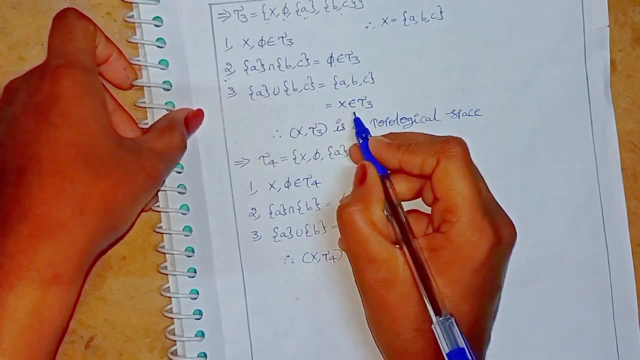 best hello, a only remain non Yorkshire, my old tutorial out of Gurling. I am telling you one of the other topography of my class c. Therefore, x equals to a, b, c. What is x, a, b, c? x belongs to tau 3.. So algebra.